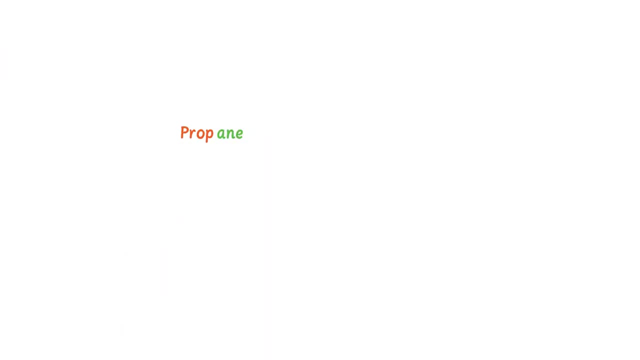 For example, consider propane: Prop means three carbons and an means, alkane. I write three carbon, I fill the four valency of carbon: H3,, H2, and H3.. Similarly, consider butane, But means four carbon and an means, alkane. 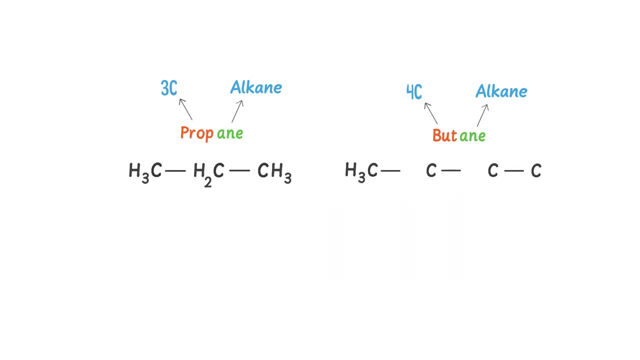 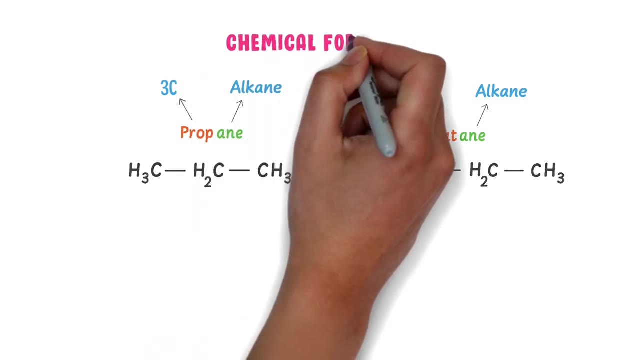 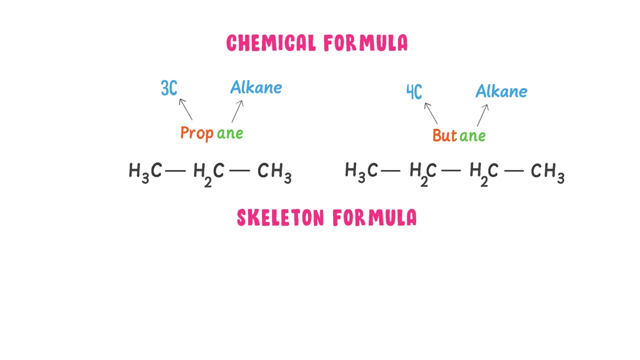 So I write four carbon. I write H3, H2, H2, and H3.. Now listen carefully. chemical formula of propane. In this lecture I will use only the skeleton formula of alkanes, For example, I will delete all the hydrogen atoms from propane. I will. 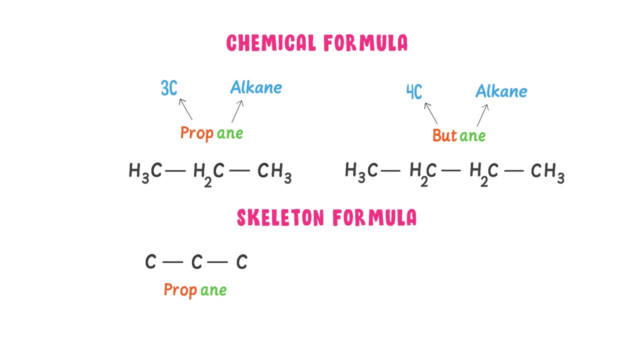 write only three carbons for propane. Similarly for butane. I will delete all the hydrogen atoms. I will write only four carbons for butane. I mean, I will only use skeleton formula for alkanes because it is easy and understandable. Now let me teach you my personal trick of 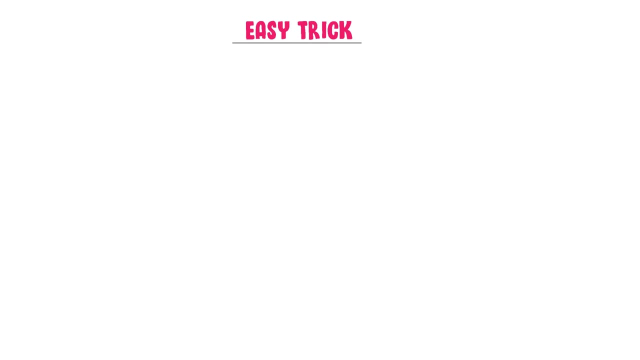 naming alkanes which you will not find anywhere. The first rule is to locate the longest father chain and son, For example. consider this alkane. Now let me locate the longest father, chain and son in this alkane, For instance, one, two, three, four, five, six, seven, eight. 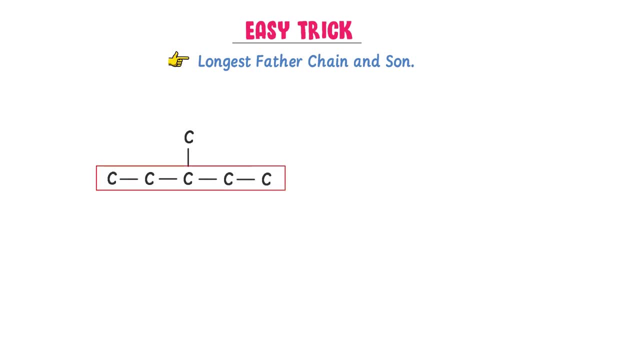 nine, ten. Now let me locate the longest father chain and son in this alkane. For instance, one, two, three, four, five, nine, ten and five. In this chain there are five carbon atoms. Similarly, one, two, three and four In this chain there are 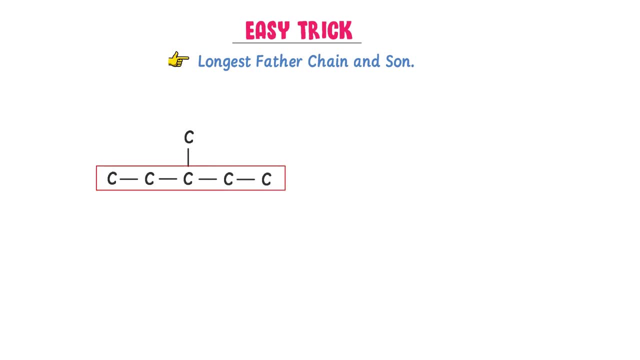 four carbons. So I select this chain as a father chain, because there are five carbons present, and eight. What about this carbon? Well, personally, I say that this is the son of this father chain. Thus, this is the father chain and this is. 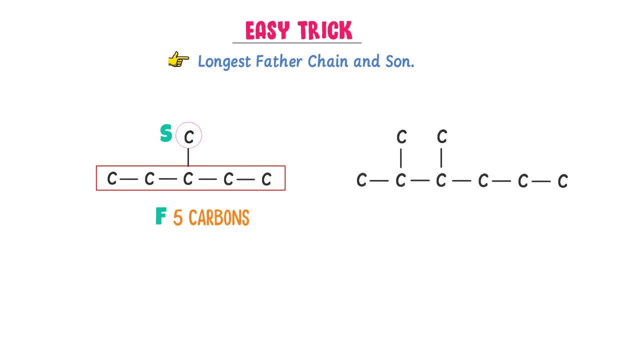 his son. Secondly, consider this: alkan: 1,, 2, 3.. There are only 3 carbons present in this chain. I skip it. Similarly, 1,, 2,, 3, 4.. There are only 4 carbons present in it. I also skip it. Similarly. 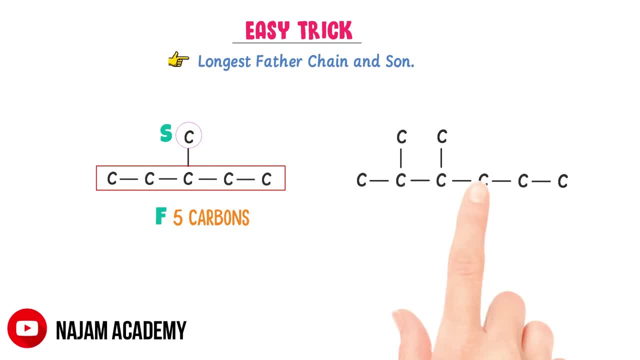 1,, 2,, 3,, 4,, 5 and 6.. There are 6 carbons present in this chain, So this is the father chain. What about this carbon and this carbon? Well, this is one son and this is another son, So this: 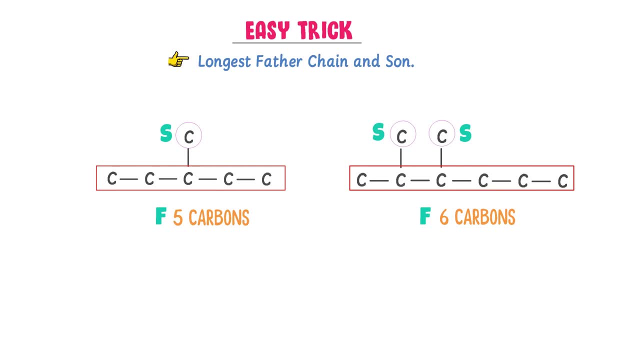 is the father chain and these are his two sons. Thirdly, consider this alkan: 1, 2,, 3,, 4 and 5.. There are 5 carbons present in it. I skip it: 1,, 2,, 3,, 4,, 5 and 6.. There are 6 carbons present. 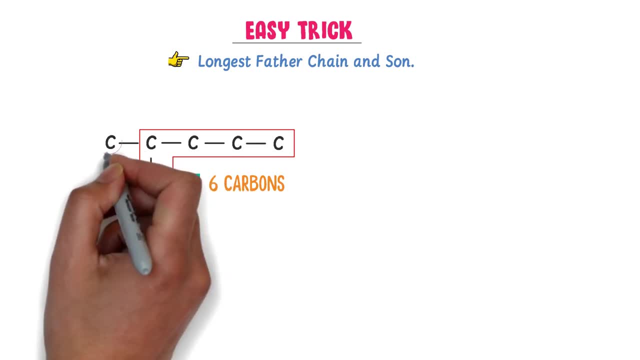 in this chain. So this is the father chain and this one, carbon, is his son. Fourthly, consider this alkan 1,, 2,, 3,, 4,, 5 and 6. I skip this chain of carbon. 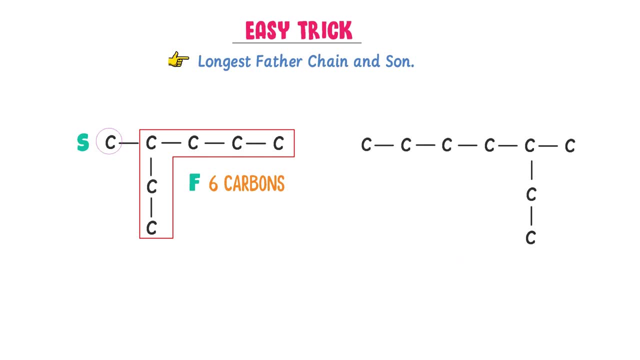 Similarly 1,, 2,, 3,, 4,, 5,, 6, 7.. There are 7 carbons present in this chain of carbon, So this is the father chain and this one carbon is his son. Fifthly, consider this alkan No 1,, 2,, 3, 4.. 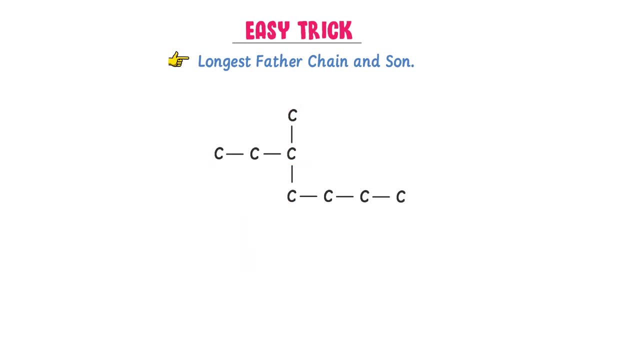 I skip this chain of carbon, Similarly 1,, 2,, 3,, 4., 5, 6.. I also skip this chain of carbon, No 1,, 2,, 3,, 4,, 5,, 6, 7.. There are 7 carbons present. 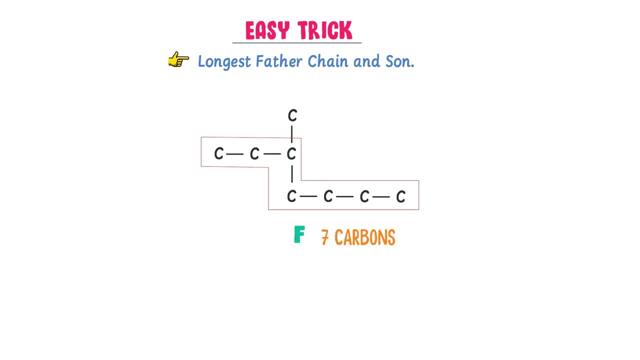 in this carbon chain. So this is the father chain and this one carbon is his son. Thus we have learned locating the father chain and his sons. The second rule is numbering the father chain And remember that. Say that now, sitting somewhere there, the father brings the son nearer, For example, 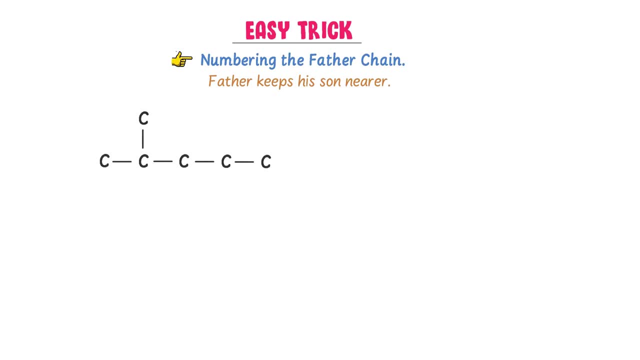 consider this, alkan. As we learned in the previous slide about the father chain and his sons, we will firstly locate the father chain and his sons While 1,, 2,, 3,, 4, and 5.. So this is the father chain and this is his son. 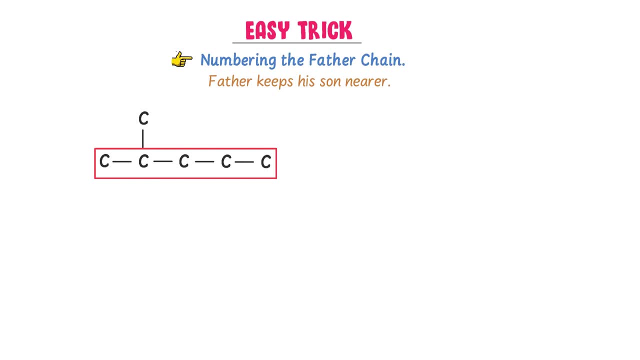 Now listen carefully. I numbered the father chain from both sides. Let me repeat it – I. I number the father's chain from both sides like 1, 2, 3,, 4, 5,. similarly, 1,, 2,, 3, 4,. 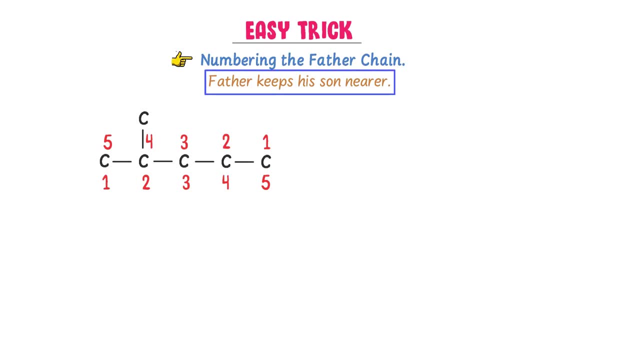 5. As I told you, that father keeps his son nearer, so in this order the son is at the 4th position, while in this order the son is at the 2nd position. So which order should the father pick? Well, he will pick this order, because in this order the son is located at the 2nd position. 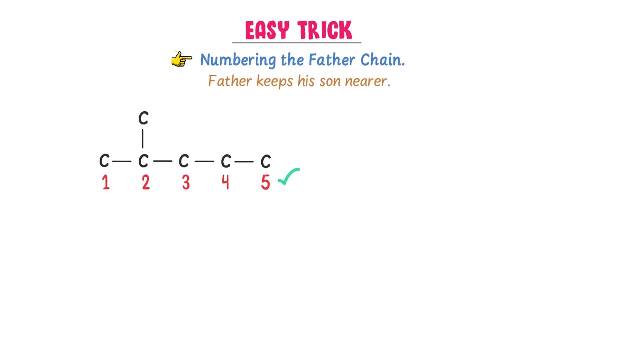 and the father keeps his son nearer. Now it is time to name this alkan. In the father chain there are 5 carbons. I write pent. all the bonds are single. I write an. so the father chain is pentan. 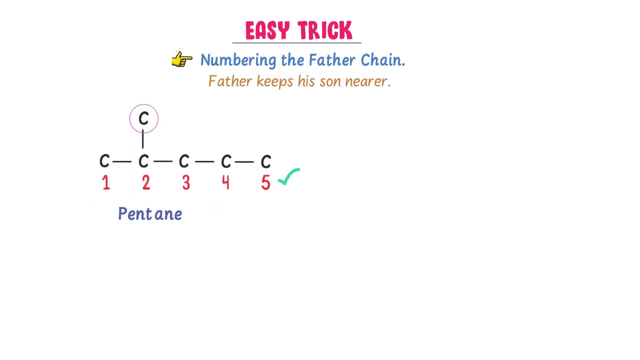 What about the son's part? Well, this is only one carbon And we call it methyl. Where is the son located? We know that it is located at the 2nd position, So the son is 2-methyl. Now, to name this alkan, firstly we write the son's part and then we write the father's. 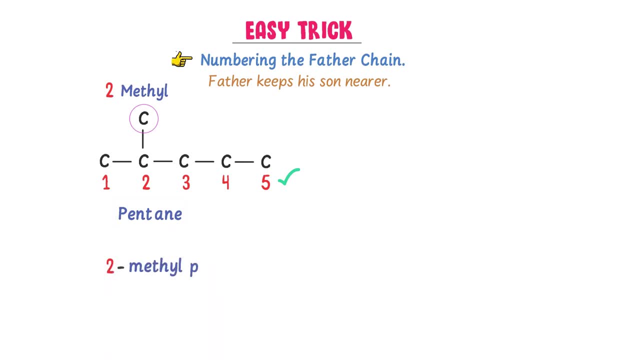 part: 2-methylpentan. Remember that before 2013 it was convention to write the first letter as a capital letter, But in 2013 it is changed: We write the first letter as a small letter. So this whole thing is 2-methylpentan. 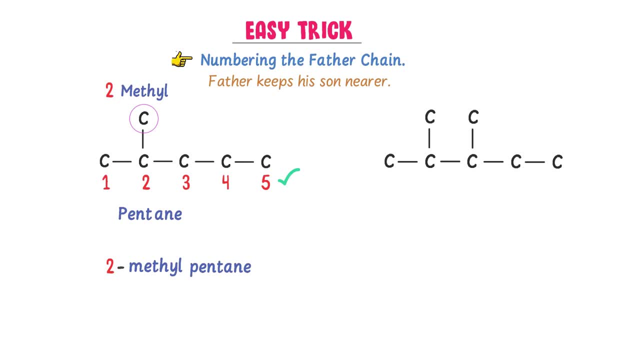 Secondly, consider this alkan. I look at the father chain and his son: 1,, 2,, 3,, 4 and 5. There are 5 carbons present in this carbon chain, So this is the father chain. 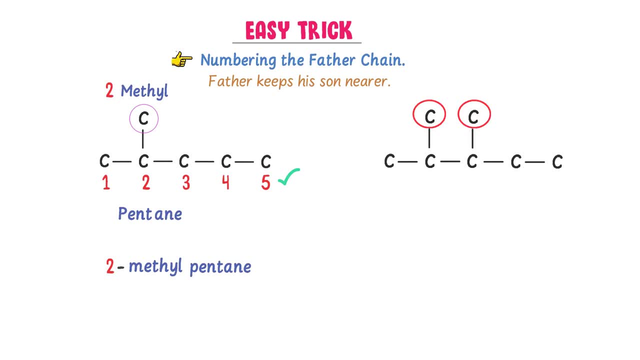 This carbon And this carbon. These are the two different sons of the father. Now number the father chain: 1,, 2,, 3,, 4, 5.. Also 1,, 2,, 3,, 4, 5.. 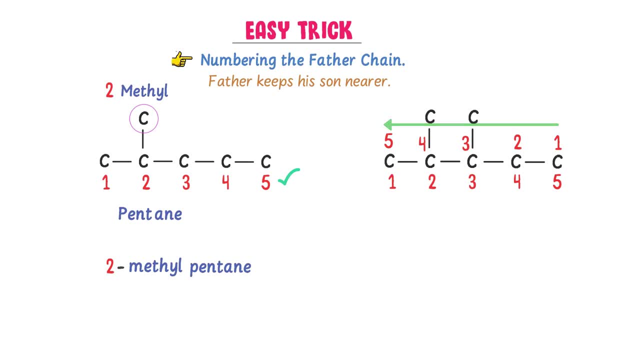 In this order, the first son is located at the 3rd position, While in this order, the first son is located at the 2nd position, As we know that father keeps his son nearer. So which order will father select? Well, he will select this order. 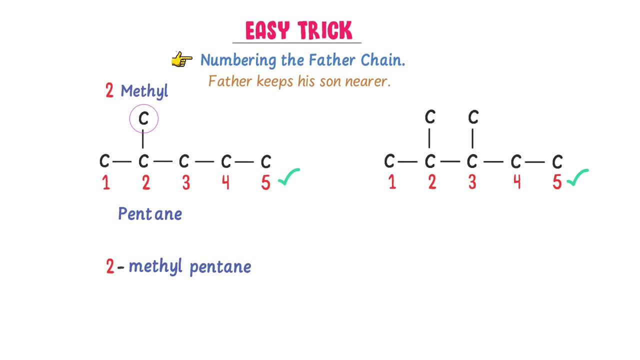 Because the first son is located at the 2nd position. Now I name the father's part and the son's part. There are 5 carbons present in the father chain. I write pent. All the carbons are single. I write an. 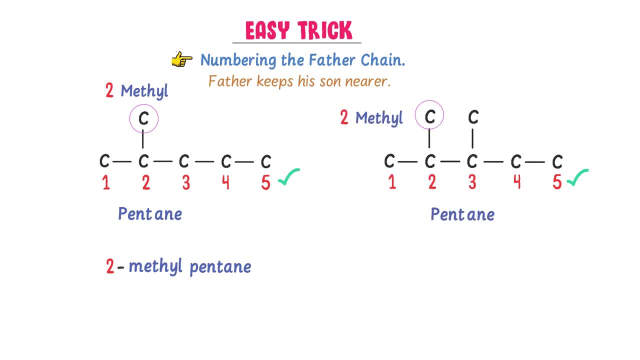 This son is present at the 2nd position. I write 2-methyl. This son is present at the 3rd position. I write 3-methyl. Now I combine the two sons. 1 son is present at the 3rd position. 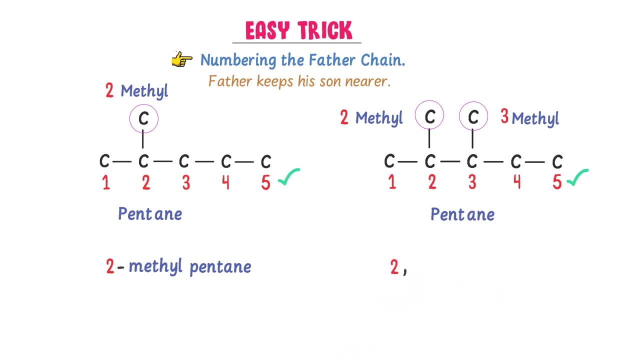 At the 2nd position. the another son is present. at the 3rd position. I write dimethyl, because there are 2-methyls present here. Lastly, I write pentane, So I get 2,3-dimethylpentane. Thirdly, consider this alkane Now: 1,, 2,, 3,, 4, 5.. Also 1,, 2,, 3,, 4, 5.. Also 1,, 2,, 3,, 4, 5.. 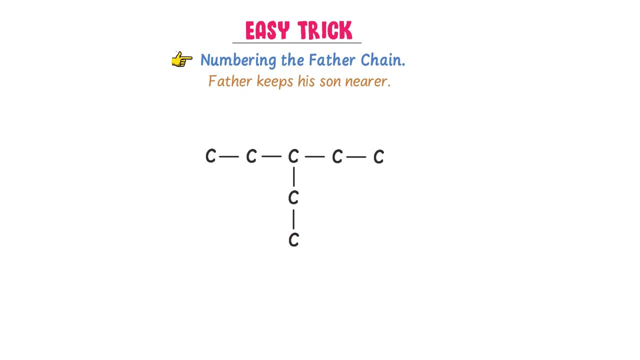 Both. the carbon chain contains 5 carbon atoms, So you can select either of them. I select this chain as the father chain and this is his son. Now I number the father chain: 1,, 2,, 3,, 4, 5.. 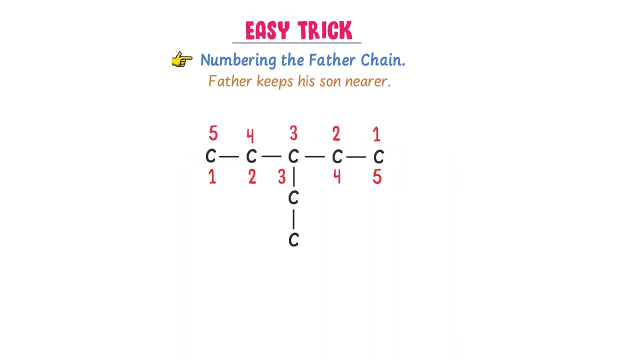 Also 1,, 2,, 3,, 4, 5.. In both the orders the son is located at the 3rd position. So father can select both the orders, Either this order or this order. Now let me name the father's part and the son's part. 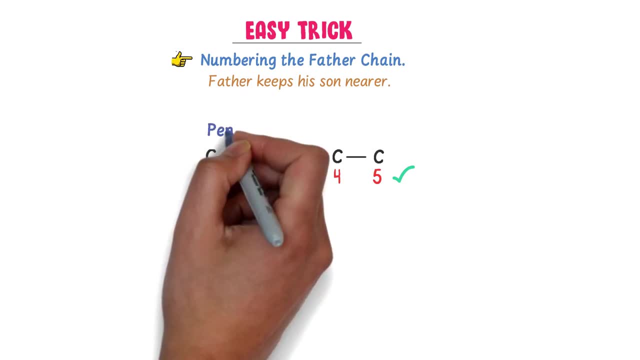 There are 5 carbons present in the father chain. I write pent. All the carbons form single bonds. I write an. The son is located at the 3rd position and his name is 3-ethyl, Thus I write 3-ethylpentane. 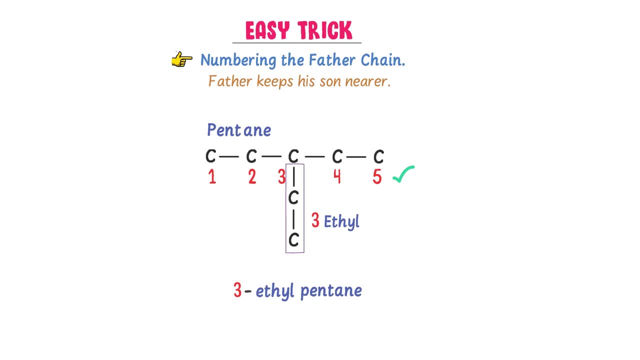 Remember that all these examples were easy. examples 1.. Now let me take you to the medium level. For example, consider this: alkan, I select the father chain and the son: 1,, 2,, 3,, 4,, 5,, 6.. 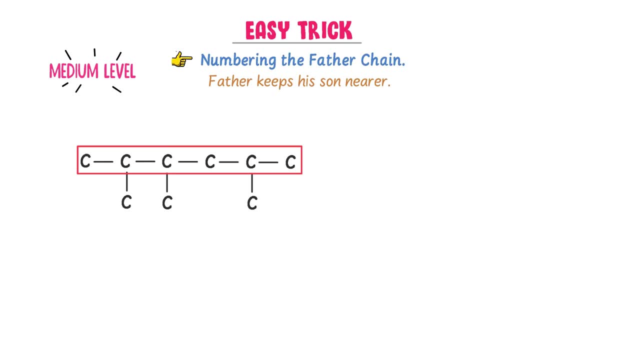 This carbon chain contains 6 carbon. So this is the father chain, This is the son, This is the son And this is also the son. Now I number the father chain: 1,, 2,, 3,, 4,, 5,, 6.. 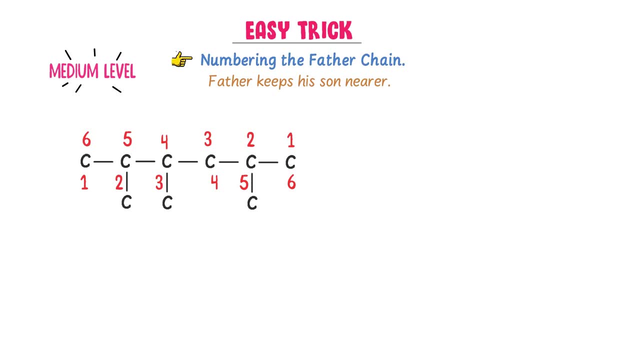 Also 1,, 2,, 3,, 4,, 5, 6.. Now, according to this order, the first son is located at the 2nd position, While, according to this order, the first son is also located at the 2nd position. 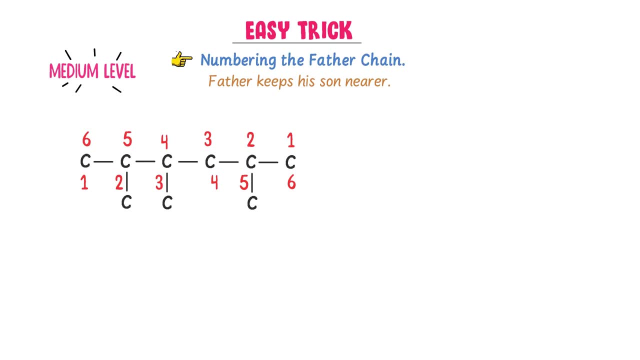 But the problem is the 3rd son. As we know, that father keeps his son nearer. Hence, which order should the father select? Well, according to this order, the first son is present at the 2nd position. Now let me take you to the medium level. 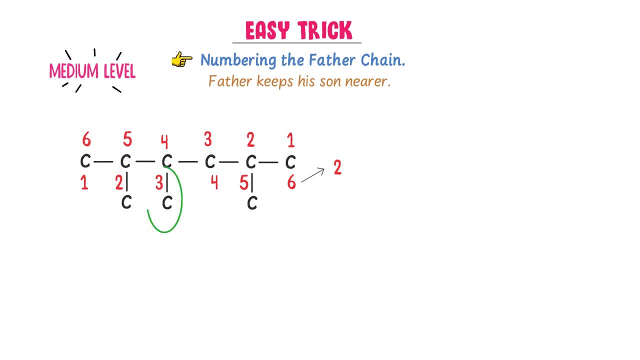 I write pent. The 2nd son is present at the 2nd position, The 2nd son is present at the 3rd position And the 3rd son is present at the 5th position, While, according to this order, the first son is present at the 2nd position. 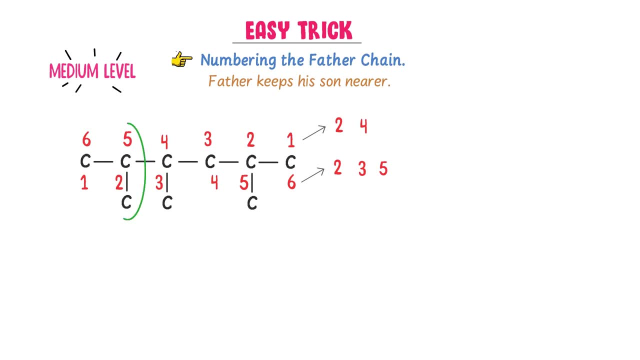 The 2nd son is present at the 4th position And the 3rd son is present at the 5th position. Now listen carefully. In both the orders the first son is present at the 2nd position, So father forgets about the 2nd position. 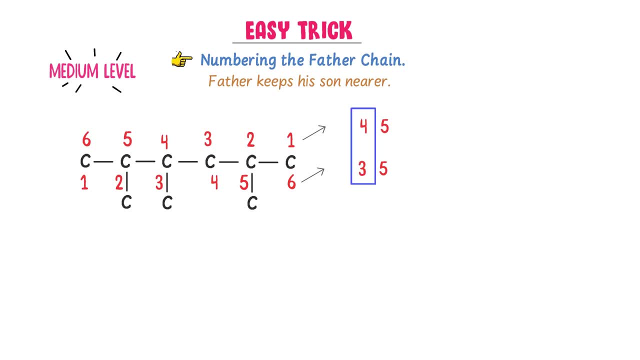 The father forgets about the 1st son. Father looks for the position of 2nd son in order to keep him nearer. In this order, the 2nd son is present at the 3rd position, While in this order, the 2nd son is present at the 4th position. 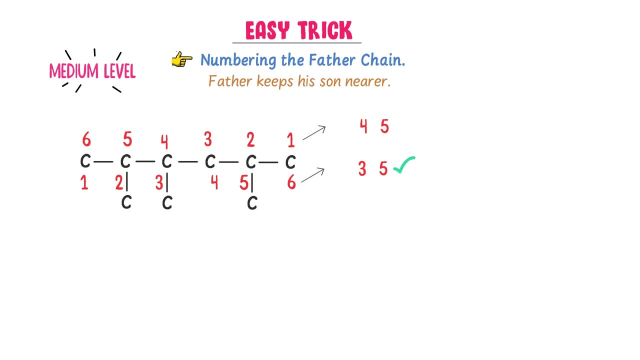 So father picks this order, not this order, Because in this order the 2nd son is nearer. Now I name father's part and son's part. There are 6 carbons. There are 6 carbons. There are 6 carbons present in father's chain. 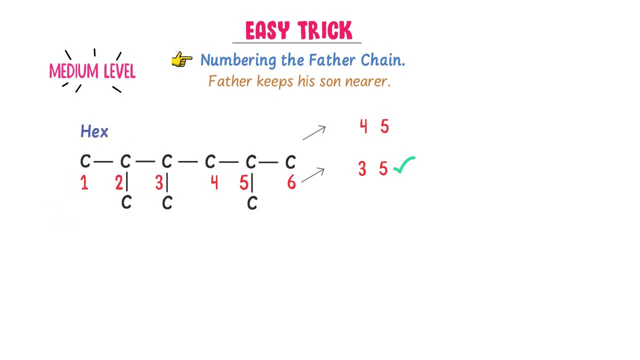 I write hex. All the carbons form single bonds. I write an. The 1st son is present at the 2nd position. I write 2-methyl. The 2nd son is present at the 3rd position. 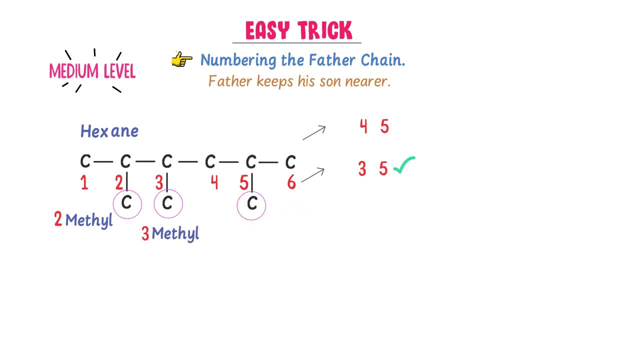 I write 3-methyl. The 3rd son is present at the 5th position. I write 5-methyl, So I write 2,3,5.. There are 3-methyls, I write 3-methyls. I write 3-methyls Hexane, Hence I get 2,3,5-trimethyl hexane. Finally, consider this alkan. I select the father chain and his son, 1,2,3,4,5,6.. 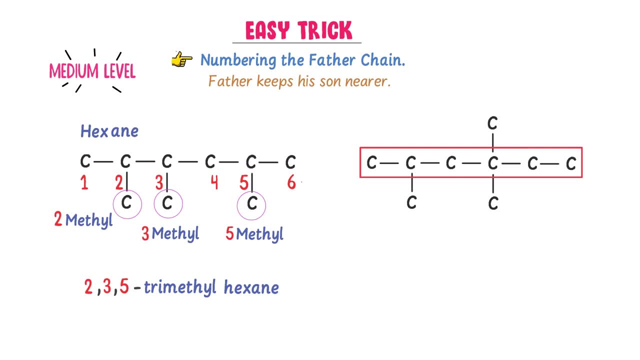 This carbon chain contains 6 carbons. So this is the father chain. This carbon is son, This carbon is son And this carbon is also son. Now I number the father chain chain: 1,, 2,, 3,, 4,, 5, 6.. Also: 1,, 2,, 3,, 4,, 5,, 6.. According to this order, the first son is present. 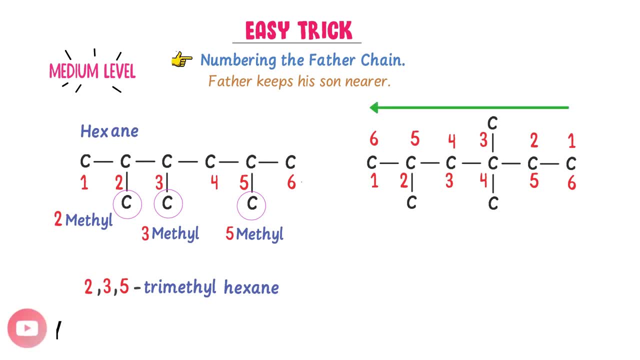 at the second position. According to this order, the first two sons are present at the third position In this order. the first son is present at second position, So father will choose this order. Now I name the father's part and the son's part. There are six carbons present in. 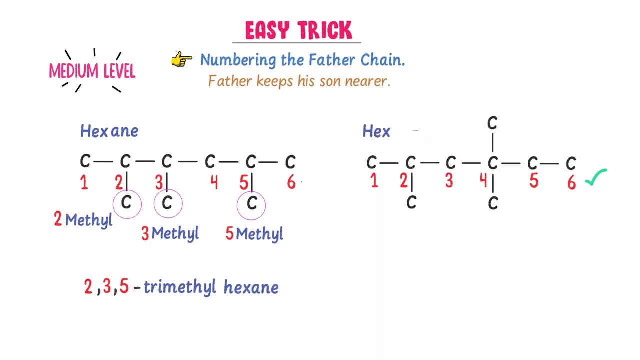 the father chain. I write hex. All the carbon bonds are single. I write n. The first son is present. at second position, I write 2-methyl. The second son is present. at the fourth position, I write 4-methyl. The third son is also present. at the fourth position, I write 4-methyl. I write. 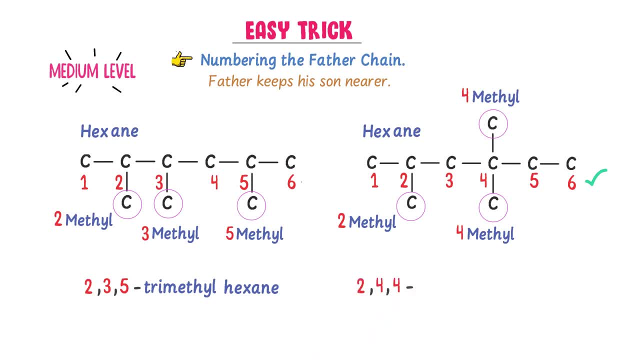 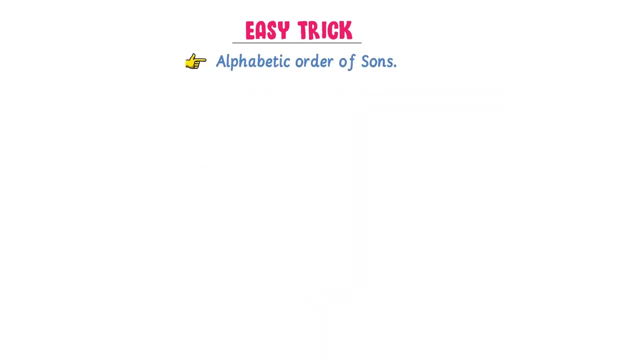 2,4,4,. there are three methyls. I write trimethylhexane, Thus I get 2,4,4-trimethylhexane. Now let me teach you the third rule. It is about the alphabetic order of suns, For example. 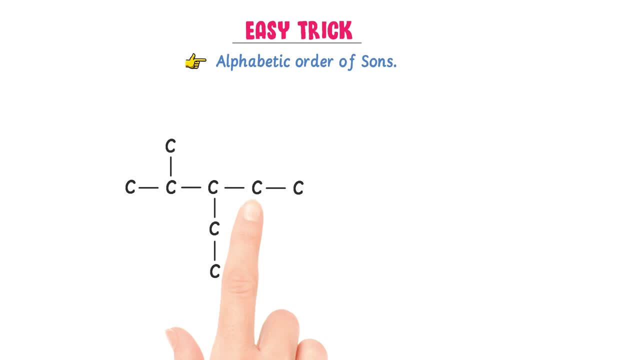 consider this: alkane: 1,2,3,4,5.. This is the father chain. this carbon is a sun and this chain of carbon is another sun. Now I number the father chain 1,2,3,4,5.. I am going to. 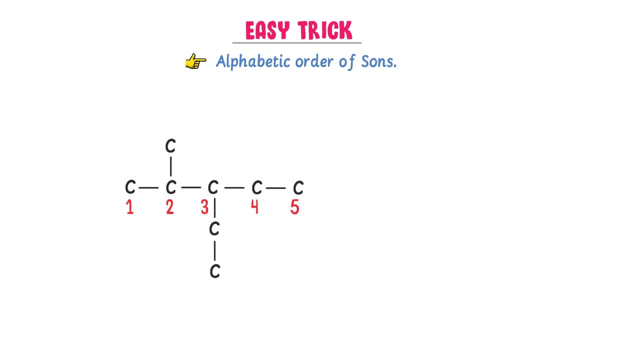 name the father's part and the sun's part. There are five carbons. I write pentane. The first sun is 2-methyl. the second sun is 3-ethyl. Now here is the problem: while writing the name of this, Alcane. 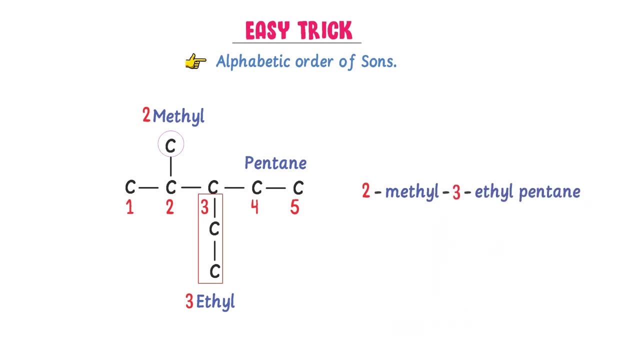 Should I write 2-methyl-3-ethyl-pentane or I write 3-ethyl-2-methyl-pentane? Well, in such cases, we follow the alphabetic order. while writing the names of the sun, We know that E comes first and M comes later. 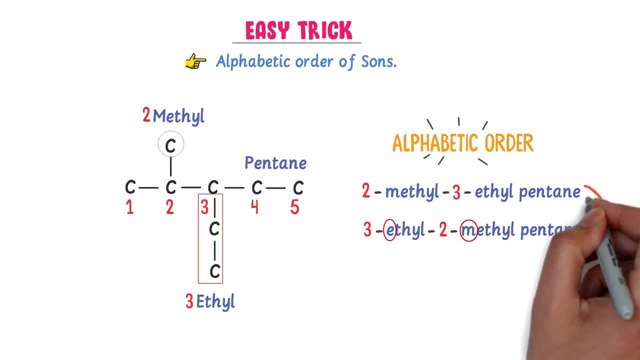 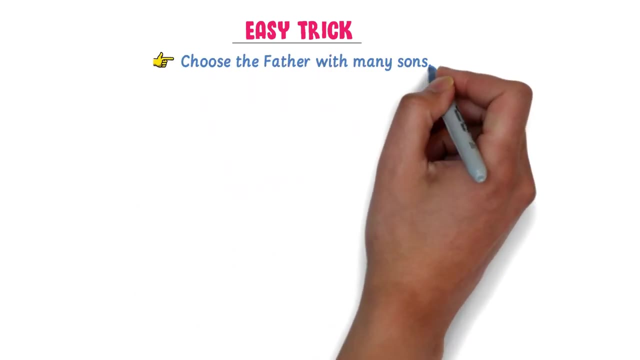 So the correct name is 3-ethyl-2-methyl-heptane. Remember that di, tri or tetra is not included in the alphabetic order of suns. Now let me teach you the fourth rule: Choose the father with many suns. 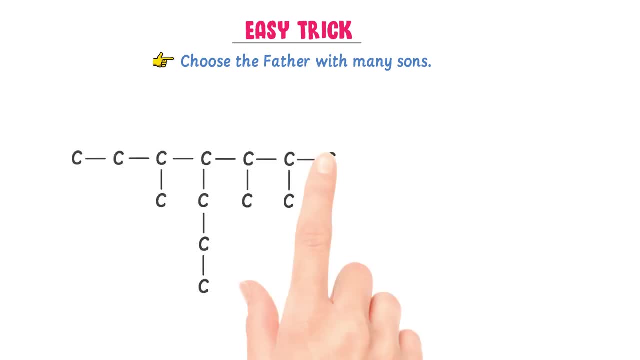 For example, consider this: Alcane Now: 1,, 2,, 3,, 4,, 5,, 6, 7.. This is one sun, this is another sun and also this is another sun, If I select this chance. 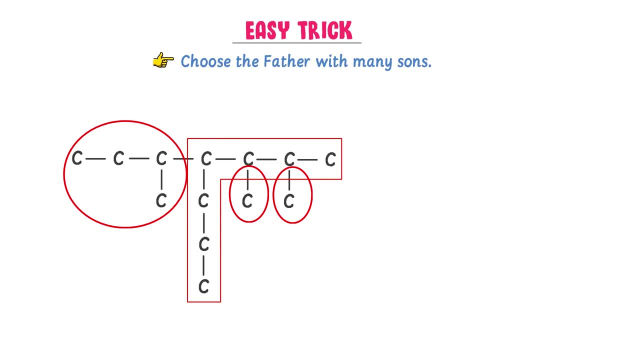 as a father chan. it has three suns. Let me try one another, chan. 1,, 2,, 3,, 4,, 5,, 6, 7.. Now one sun, second sun, third sun and fourth sun. 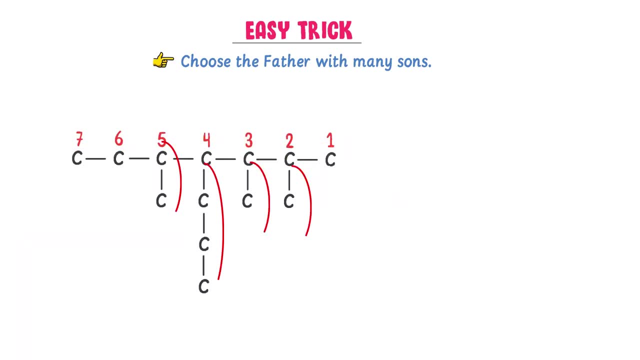 I select this chan as a father chan because it has four suns. I name the father's part. I write heptane because there are seven carbon present in this Alcane. Now I name the sun's part: 2-methyl, 3-methyl, 4-n-propyl and 5-methyl. 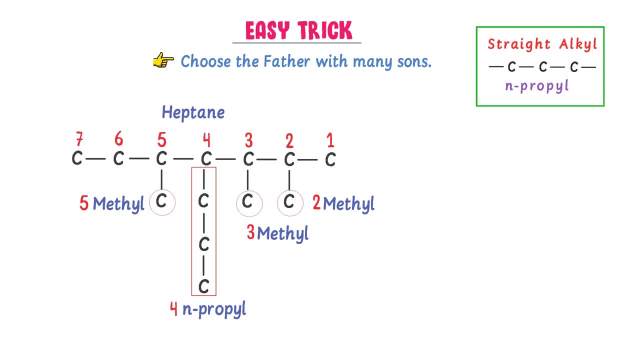 Remember that for straight alkyl, like propyl, we use n-propyl. For branched alkyl, like this butyl, we use isobutyl, Now m, and the methyl comes first from p and the propyl. So I write 2,, 3,, 5.. 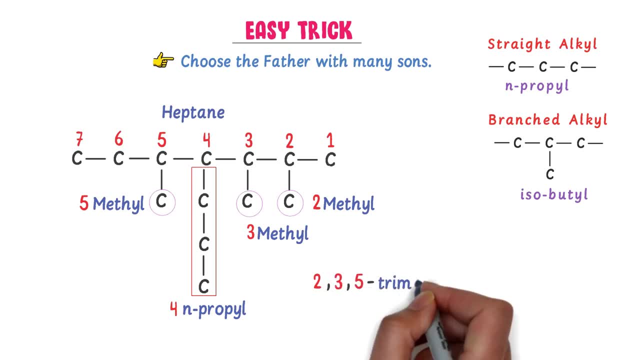 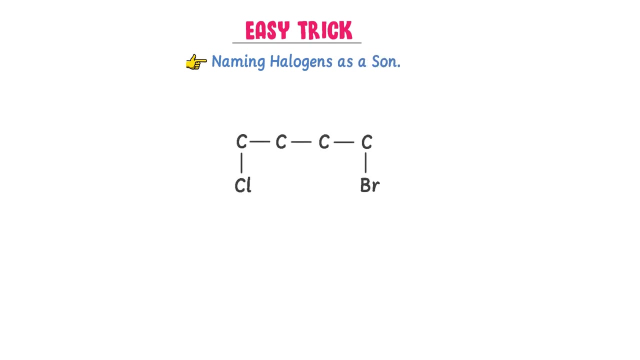 There are three methyl. I write trimethyl, then 4-n-propyl-heptane, So this is the name of this Alcane. Lastly, the fifth rule is naming halogen as a sun. Consider this Alcane. Can you name this Alcane? 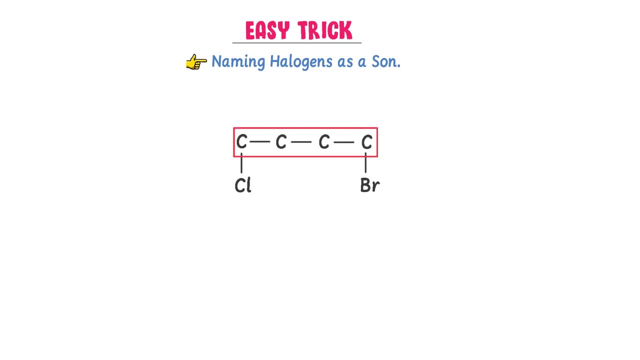 Well, this is the father chan. This chloro is the sun and this bromo is the sun. Now I number the father chan: 1, 2,, 3,, 4,, 5,, 6, 7.. 1, 2,, 3,, 4,, 5,, 6,, 7..